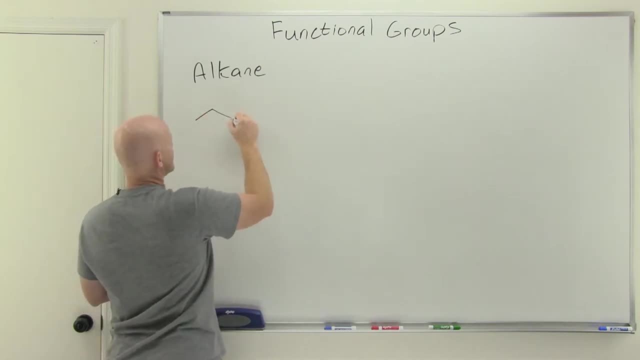 functional group and stuff. But so in this case you might have something as simple as just a four-carbon chain here. So we would call this butane- And we'll learn how to name those much later here- So, but in this case just a simple four-carbon chain. 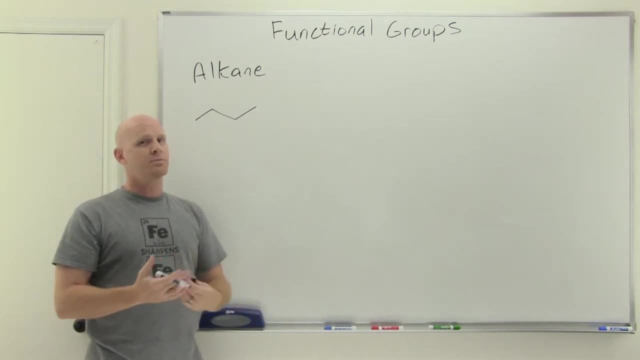 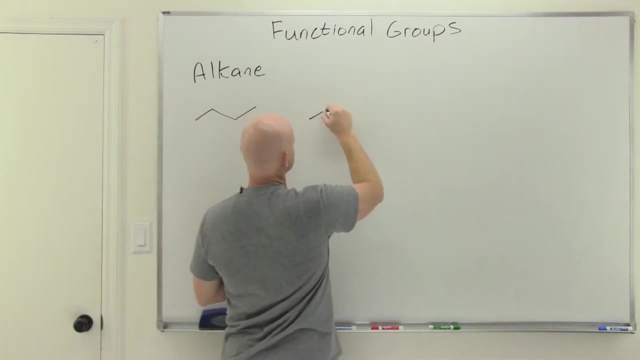 So there's no other atoms besides carbon and hydrogen, No double bonds, No triple bonds. This would be an example of an alkane. Now let's do a little more complicated example here And one more, So we'll do something looking like this here: 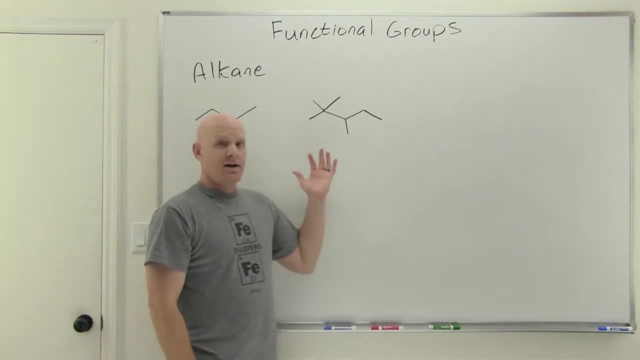 And I just want to point a few things out here. So this is not always the place where we kind of point these things out, but we often classify different carbon atoms based on how many other carbon atoms they're bonded to. So I just want to point this out. 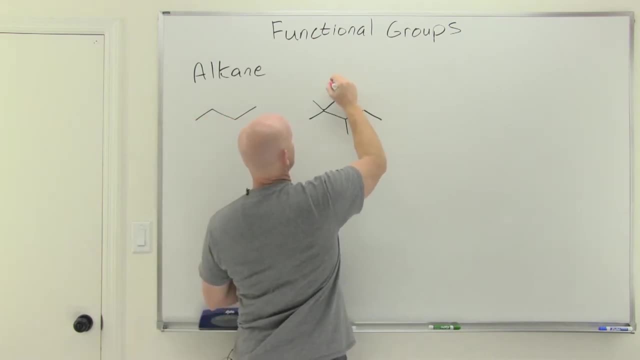 So like this carbon atom here, like this one here or this one here, or technically this one, this one or this one, So these are all carbon atoms that are bonded to only one other carbon, And this might be. 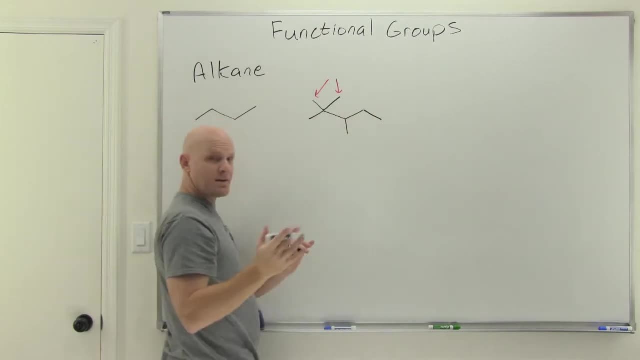 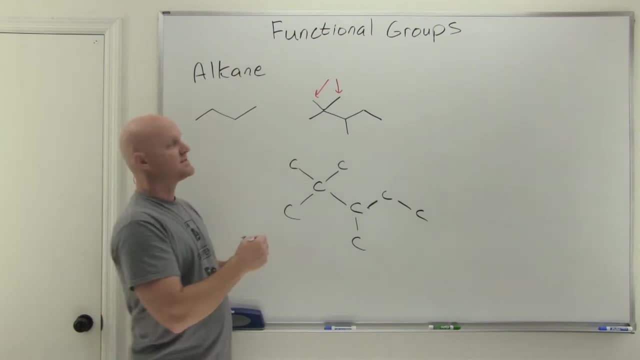 they're all directly only bonded to one other carbon, And so we would refer to those as primary. So, and we often use this little one with a degree symbol to represent primaries, That's the symbol for primary, And again, a primary carbon atom would be a carbon atom that's bonded directly only. 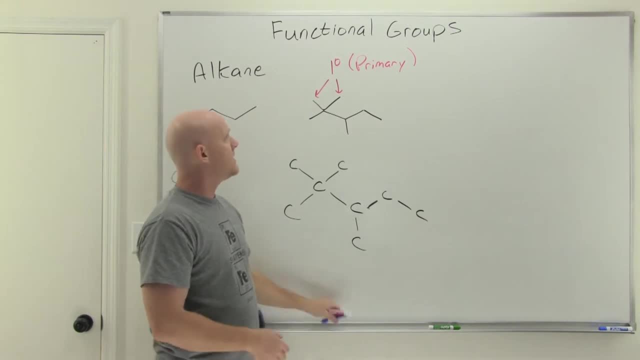 to one other carbon atom. Okay, So let's move on here. So we've got this guy right here. This carbon atom right here which is represented by this one is directly bonded to two carbon atoms, And we refer to him as being secondary. 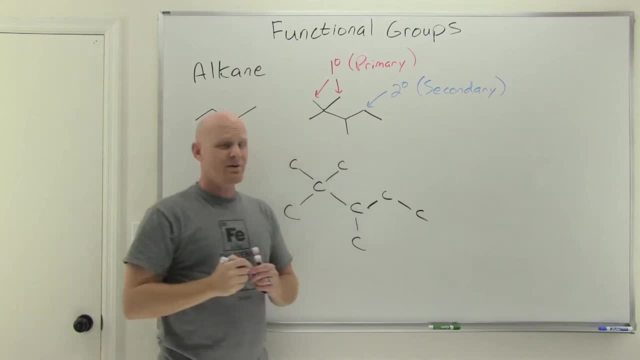 Cool, And that's a secondary carbon atom, So we'll move on here. And in this case we've got this carbon atom right here, which is representing this one right here, And it's directly bonded to one, two, three other carbon atoms. 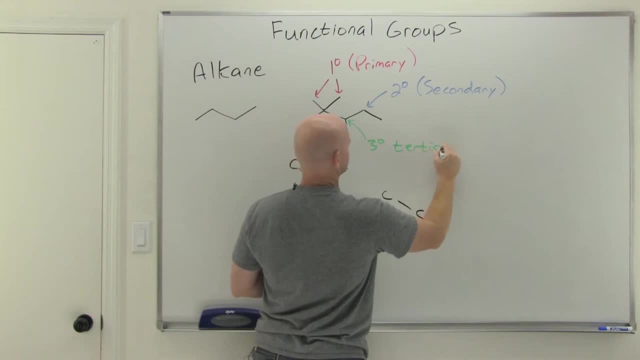 And so we refer to him as being tertiary. So, and then finally- and I'm out of color, so we'll just repeat, Maybe we'll just do black. So we've got this carbon atom right here, Okay, Okay. 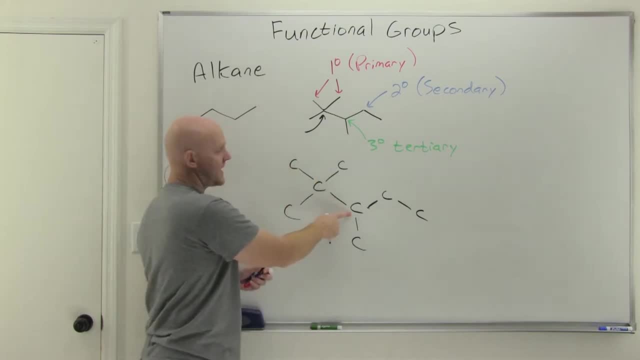 Which is this one right here, And it's directly bonded to one, two, three, four other carbon atoms. So all four of this carbon's bonds are all to carbon atoms And we refer to him as being quaternary, which is a little four-degree symbol. 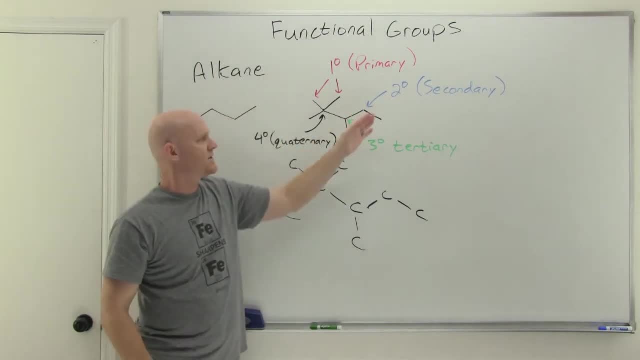 Cool. And those are the four different types of carbons. So we've got primary, secondary, tertiary, quaternary, And this will be an important designation. We'll find out that a lot of the different functional groups will have similar designations. 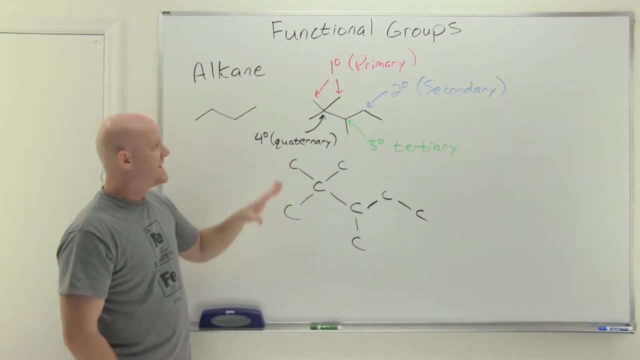 So- and we'll see kind of how it relates to this kind of terminology here- So in addition to being able to give these carbons such rankings- primary, secondary, tertiary, quaternary- we can also give the hydrogens on this molecule the same kind of thing. 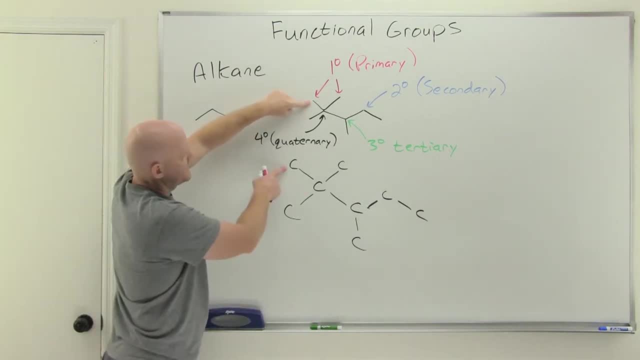 So if you notice, like this carbon right here, which again represents this carbon right here, So only got one bond showing. So with only one bond showing, it should have three other bonds to hydrogens. So I'm just going to draw one of those hydrogens in. 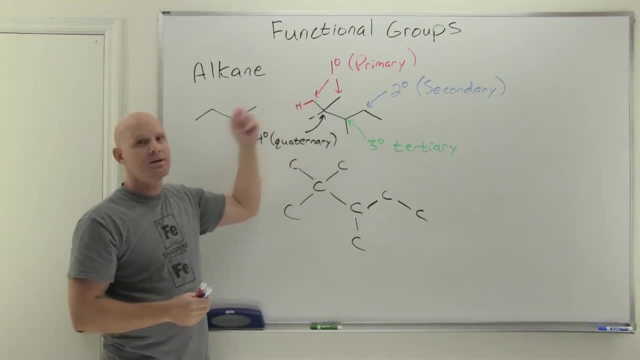 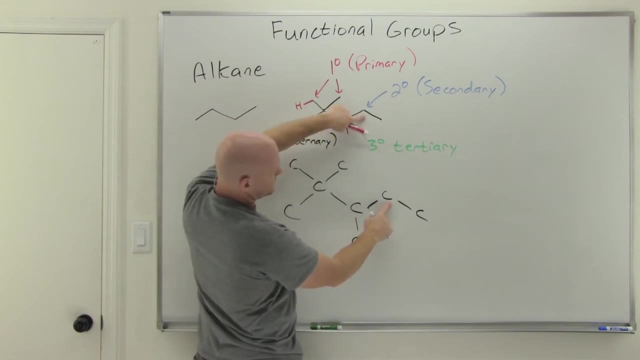 So, but a hydrogen that's attached to a primary carbon is referred to as a quaternary. So in similar fashion. so this carbon right here, which again represents this one right here, So it's got two bonds showing, So it has two bonds to hydrogens. 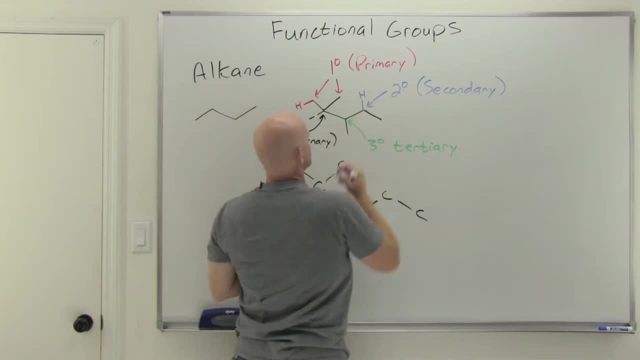 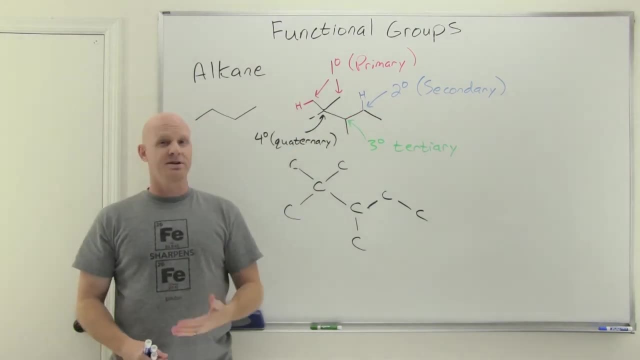 And again I'm just going to draw one of those hydrogens in. So, and either one of those hydrogens on a secondary carbon would be referred to as a secondary hydrogen. A tertiary hydrogen would be a hydrogen attached to a tertiary carbon. 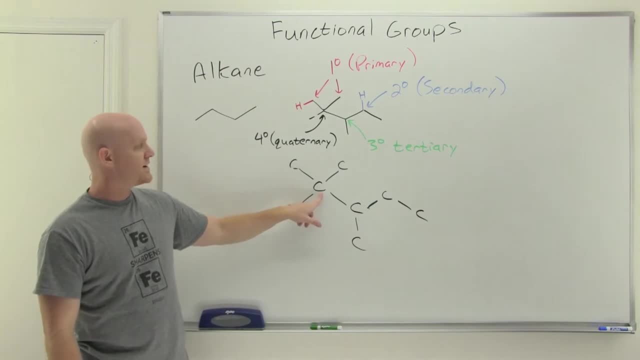 And then there's no such thing as a quaternary hydrogen. So, because if you're a quaternary carbon, you have no room for any hydrogens. So there's no such thing as a quaternary hydrogen. But so we've got primary, secondary and tertiary hydrogens are just simply hydrogens. 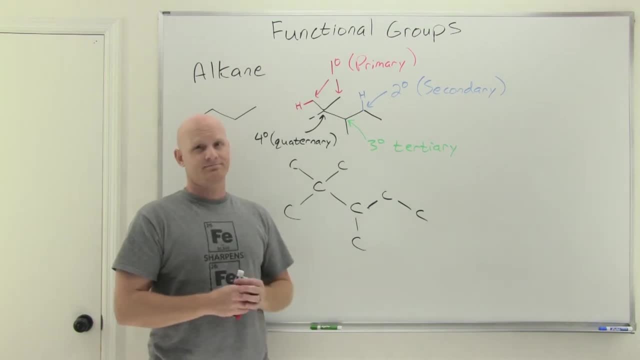 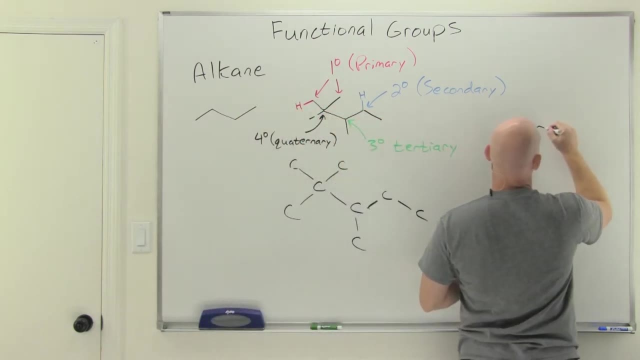 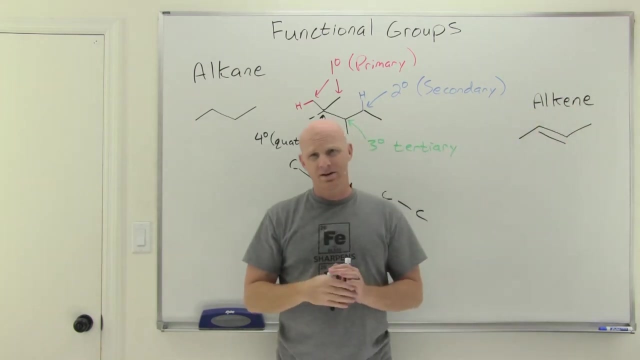 that are attached to primary, secondary, tertiary carbon atoms. Cool, Let's make this a little more challenging here. So a couple more functional groups. So another hydrocarbon here, but this time we're going to have somewhere in the structure. 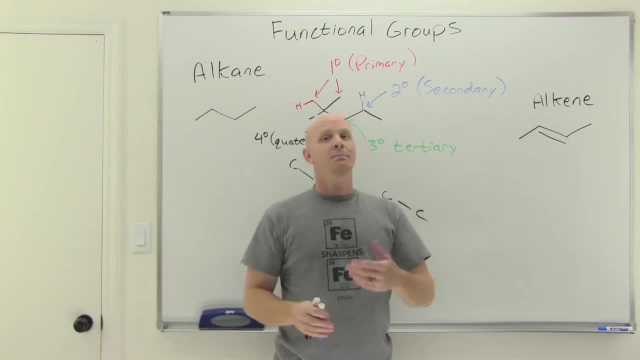 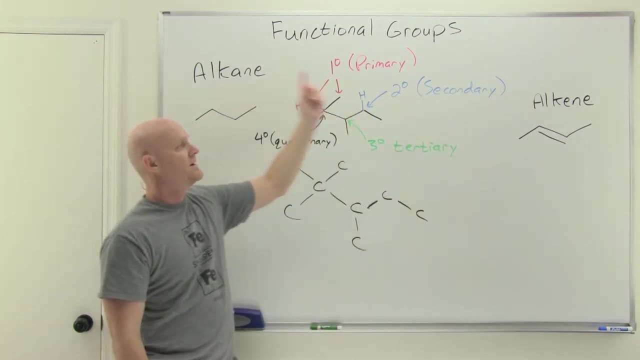 at least one carbon-carbon double bond. You can have more than one, but at least somewhere in the structure you've got to have a carbon-carbon double bond, And that is referred to as an alkene. Notice the similarity in the name alkane. 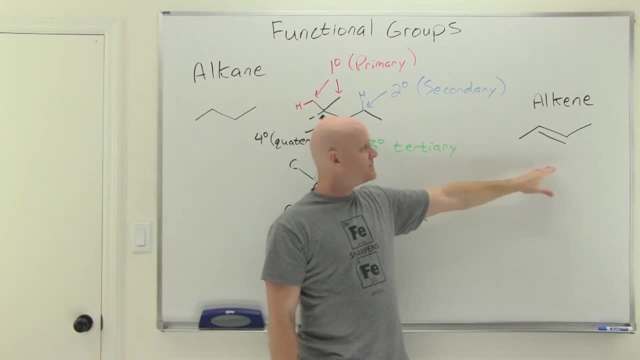 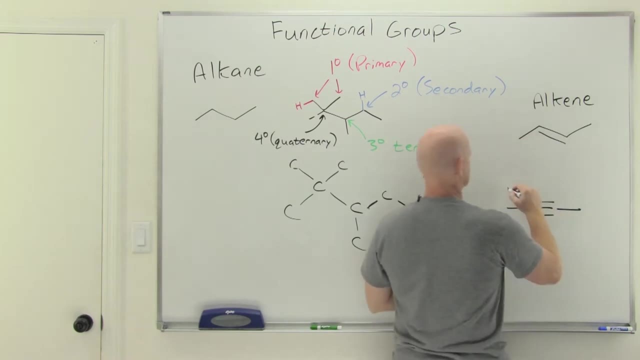 And now we're going to say: alkene, Just one letter change, but it implies that we now have a carbon-carbon double bond. In similar fashion, now we've got a carbon-carbon triple bond, And this is going to be called an alkyne. 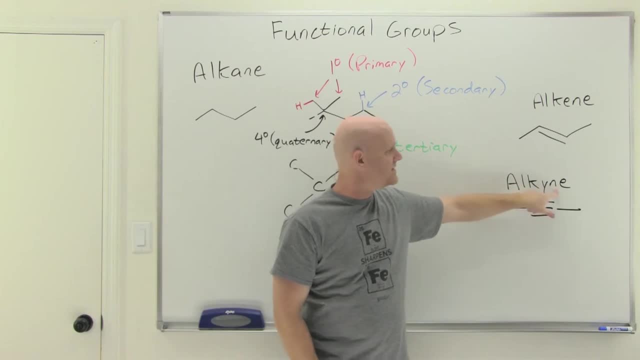 So again a one-letter change. Now we'll change that letter right in between the K and the N to a Y, alkyne. And now we've got a carbon-carbon triple bond. So alkanes, alkene. 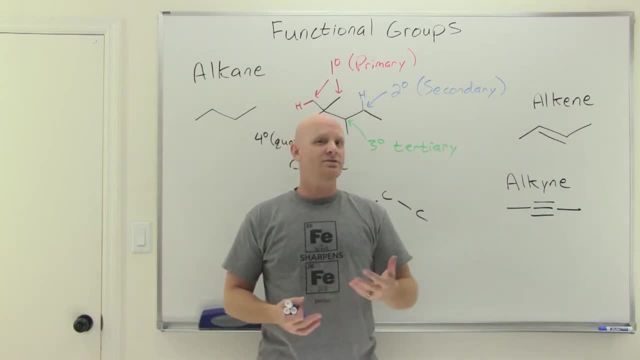 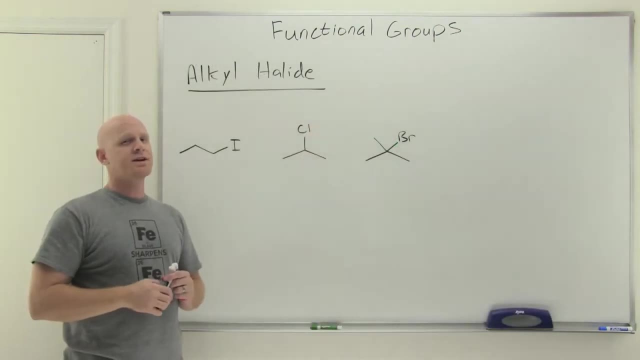 Alkynes, alkynes- They're all hydrocarbons, It's just: do we have a carbon-carbon double or triple bond present somewhere in the molecule? All right, next functional group we'll take a look at is an alkyl halide. 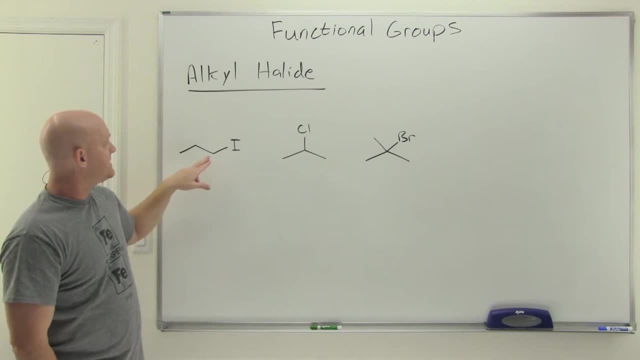 So an alkyl halide. here is where you've got an sp3 hybridized carbon here. So this carbon bonded to four things, So two hydrons, a carbon and an iodine here, So bonded. But one of those bonds is to a halogen. 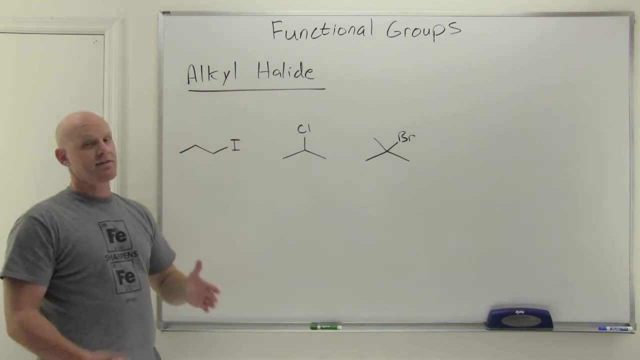 So to be a halide, you've got to have, in this case, first off a halogen- Fluorine, chlorine, bromine iodine- And to be an alkyl halide, So the halogen's got to be attached to an sp3 hybridized carbon. 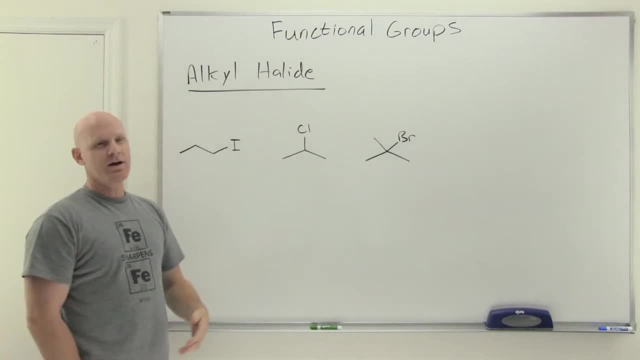 Sometimes we might call it an alkane carbon. You might think of it that way. So we just learned that. functional group, So, but short for alkane. here is this: alkyl instead. So, but alkyl halide. So each of these is an example of an alkyl halide. 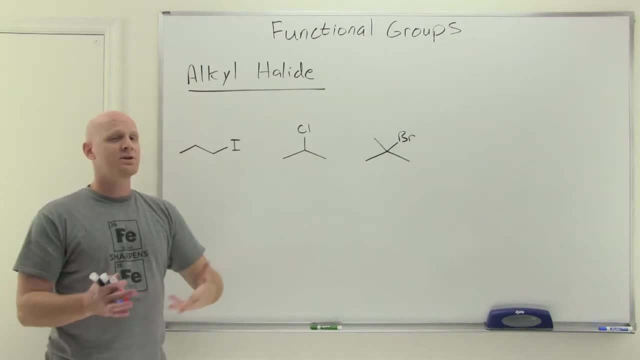 So, and just like we can rank hydrogens as primary, secondary, tertiary, depending on if they're, you know, the carbon they're bonded to, we rank halides exactly the same way. So in this case, This alkyl halide. 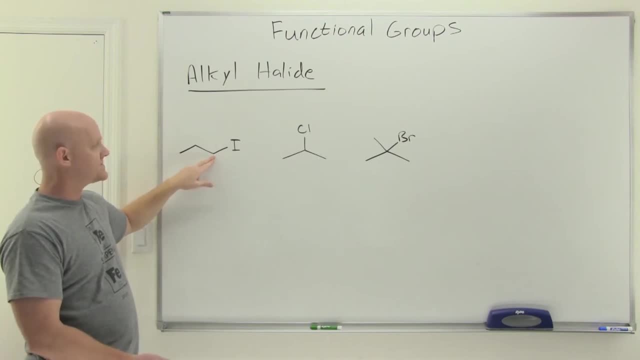 The halogen's attached to this carbon. And this carbon right here is only bonded directly to one other carbon. So keep in mind, there's your carbon skeleton. So this carbon right here is only bonded to one other carbon. It doesn't matter what everything else it's bonded to. 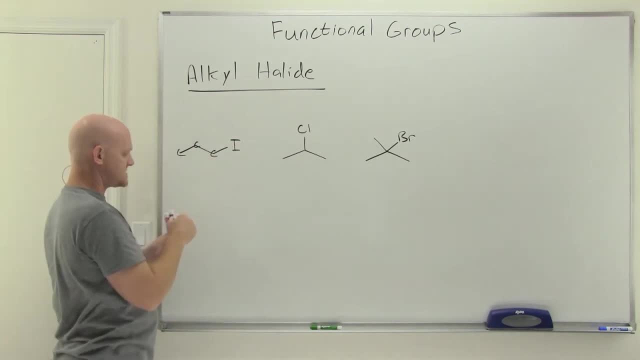 Hydrogens, halogens, whatever, But that carbon's directly bonded to only one other carbon, So we would refer to this guy as a primary alkyl halide. So again for halogens, it's based on the carbon. 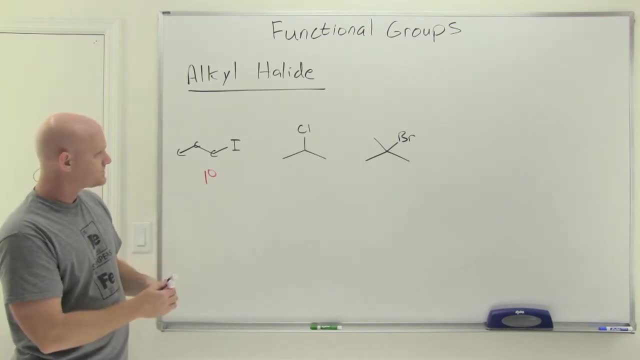 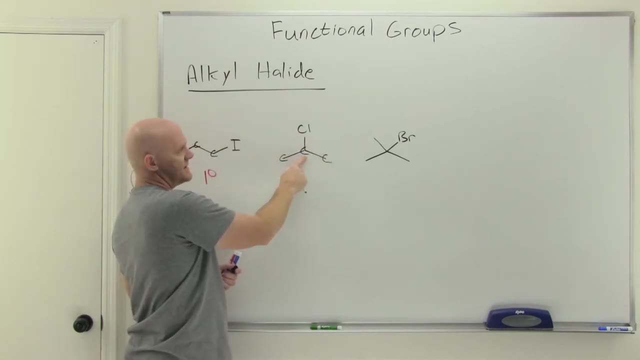 The halogens attach you, just like we saw with hydrogen atoms. Cool, This one right here. show that carbon skeleton again. So the carbon attached to the halogen is now bonded directly to two other carbons, And so, since the halogen's attached to a secondary carbon, we would refer to this. 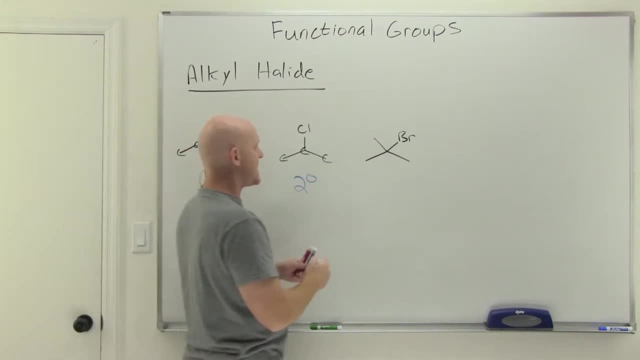 as a secondary halide. And then finally, in this last one again, we'll highlight all the carbons. And so now the halogen is bonded to a carbon atom that's directly bonded to three other carbons, And so we'll refer to this as a tertiary alkyl halide. 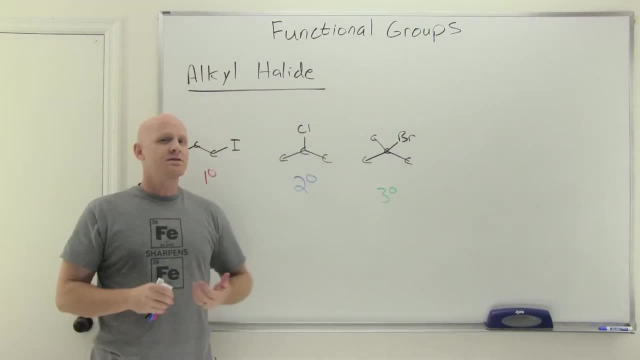 So- and this comes down to some importance that we'll see towards the end of this first semester- So it turns out, whether you're a primary alkyl halide, a secondary alkyl halide or a tertiary alkyl halide, that'll give you some differences in chemical reactivity and 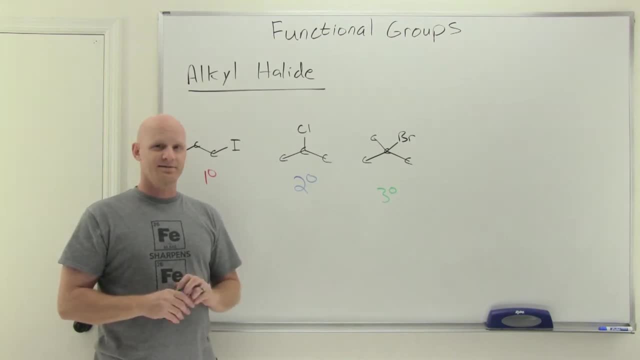 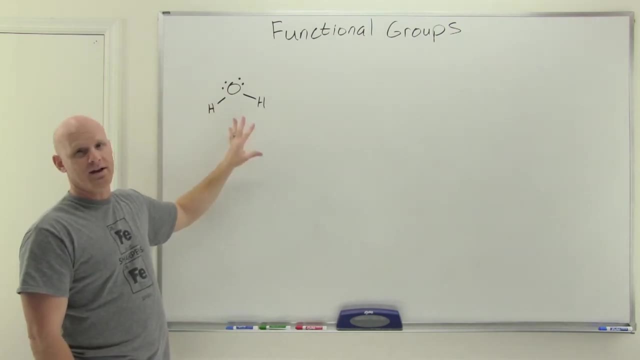 some certain reactions. we'll definitely spend a whole chapter studying. All right. Now I want to talk about a couple of oxygen-containing functional groups, And we're going to start with water. Obviously, this is not an organic molecule, So, but I want to start with this as the base because we're going to replace first one of 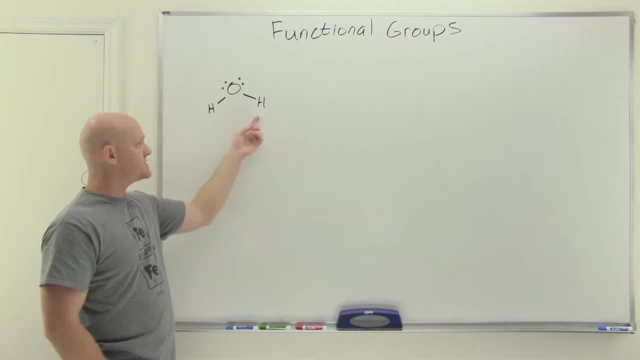 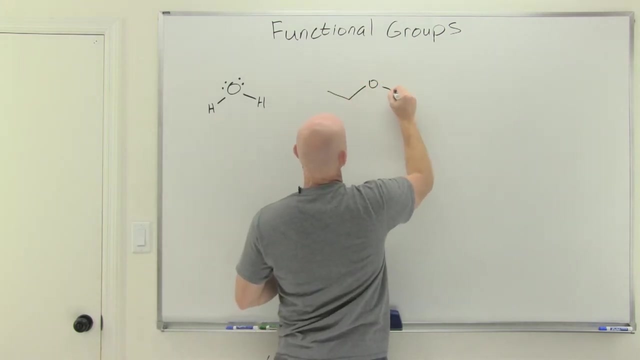 these hydrogens with a carbon chain And then we'll replace both of those hydrogens with carbon chains to get two new functional groups. So first thing we'll do is replace one of the hydrogens with a carbon chain And the functional group that results is called an alcohol. 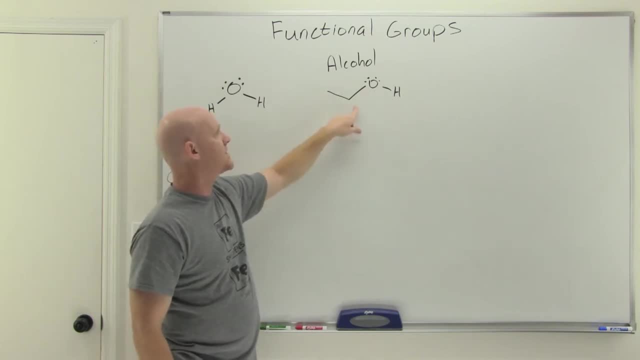 And so the key is, you got to have an oxygen bonded to one hydrogens and then one carbon chain. So there's one example, There's another example And yet a Another example here. Let me get those lone pairs drawn in. 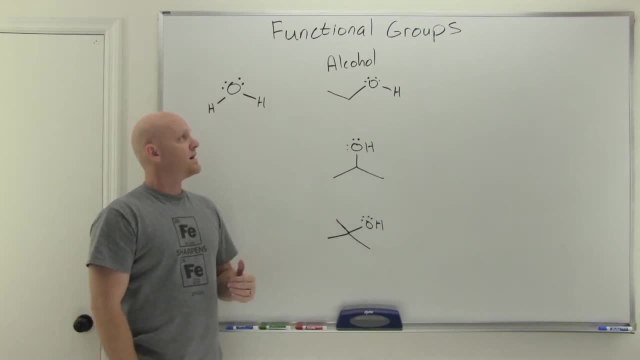 All right, So I've drawn three examples here. So, but it turns out alcohols have a most famous member, And that most famous member is ethyl alcohol, or ethanol. That's the drinking alcohol you'll find in fermented fruits and stuff like this. 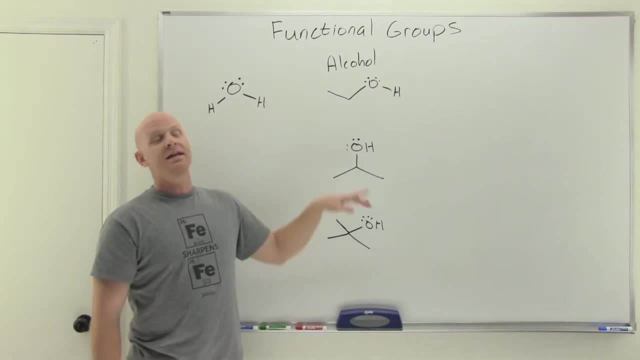 So that's this guy. So when somebody just says, hey, pass the alcohol, that's probably what they're referring to. It's the most famous member, But technically we've got hundreds of different alcohols that could exist. 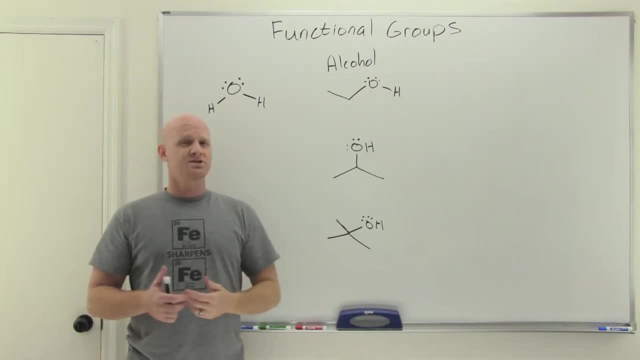 So it's kind of like the same thing you saw in general chemistry. You know, when your mom says, hey, you know, Chad, pass me the salt. Well, I know she's talking about sodium chloride, So. but if you're in the lab and somebody says, pass me the salt, 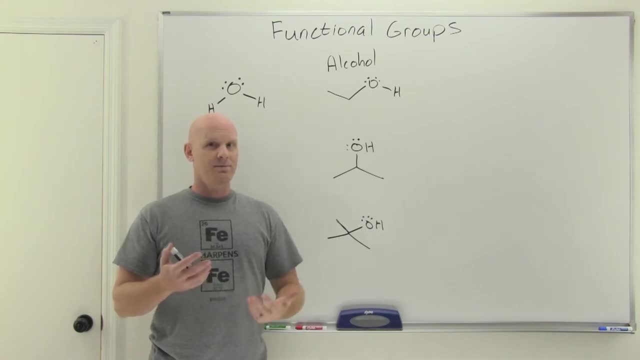 Well, in the lab I'm like, well which one? Any ionic compound can be termed a salt, So different in the kitchen than it is in the laboratory, And so same thing here. You know, if you're out with your buddies and somebody says alcohol, you probably know. 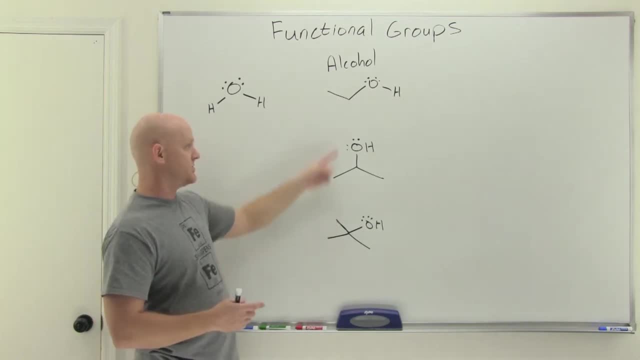 they're talking about this, But if you're in a chemistry lab and somebody says alcohol, you have no idea which of you know a few hundred different alcohols. they might be talking about Things of this sort, So, but these are all alcohols. 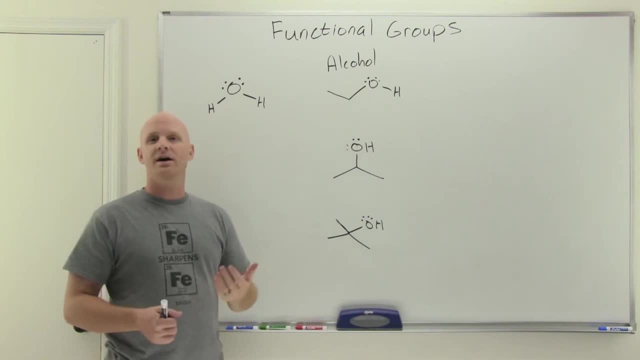 And I want to show you that we can Classify alcohols the same way we classified, you know, alkanes and alkyl halides and stuff like this. And so for an alcohol, we always classify them based on the carbon that the oxygen is. 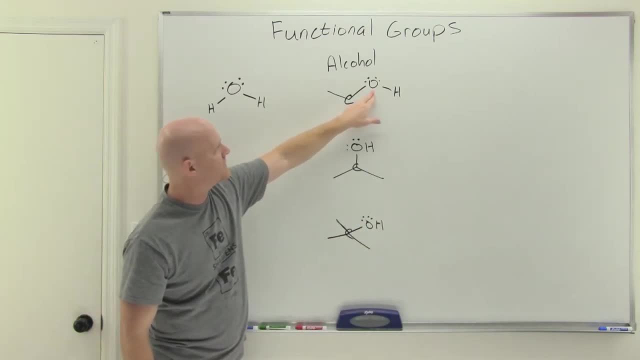 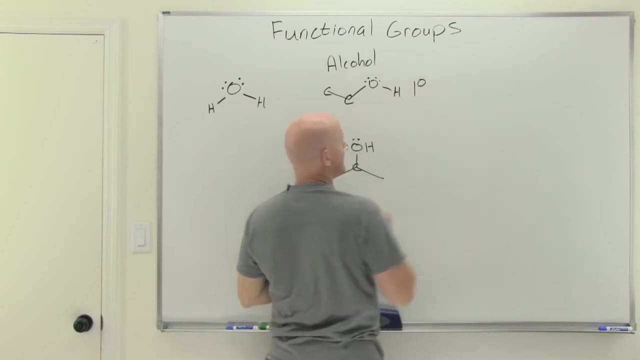 attached to, And so in this case, this carbon right here that the oxygen is attached to, so is bonded directly to only one other carbon, And so we would refer to this as a primary alcohol. So in the next example, the carbon that the oxygen is attached to is directly bonded to. 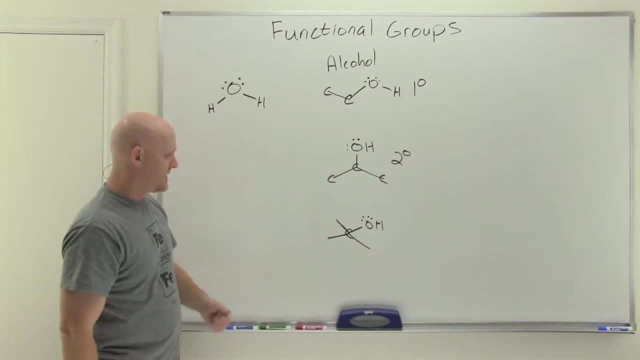 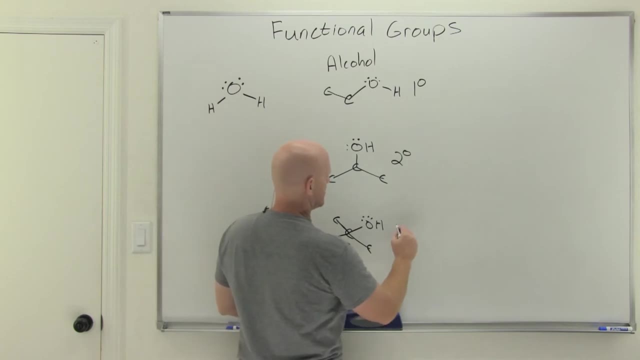 two other carbons, And so we'd call it a secondary alcohol. And then, finally, the next one: the carbon that the oxygen is bonded to is directly bonded to three other carbons, And so we'd refer to this as a tertiary alcohol. 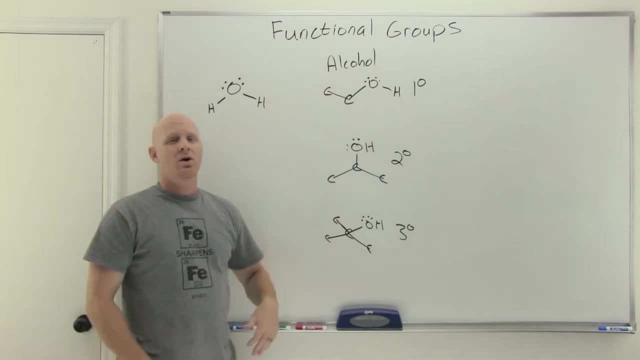 And again, we'll find out when we get to this chapter in second semester on alcohols that you'll see a difference in chemical reactivity based on these different classifications: primary, secondary, tertiary. So that's again why this is getting just a little bit of press. 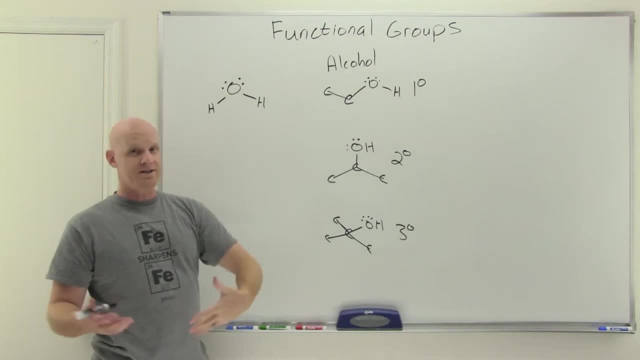 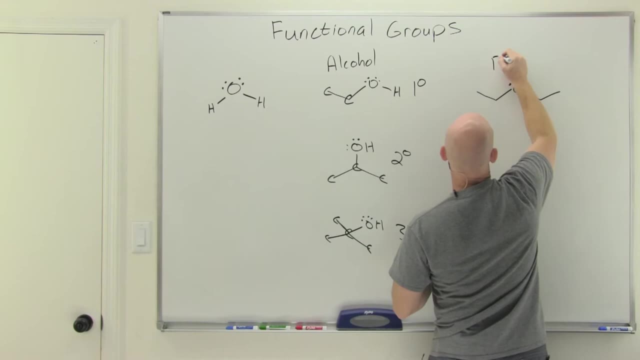 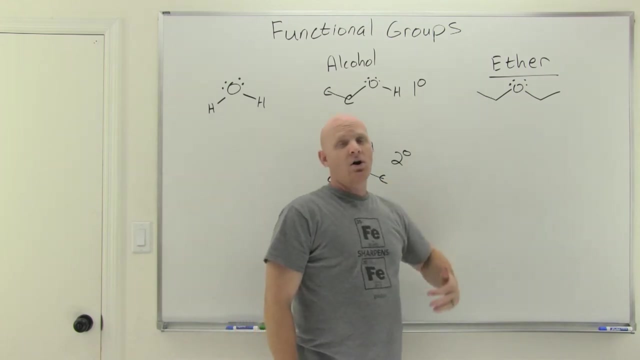 Now, if we go through and replace both of these hydrons now with carbon chains, we'll get yet A new functional group. All right. So this is called an ether now. So, and just like with alcohols, which have a most famous members, ethers have a most. 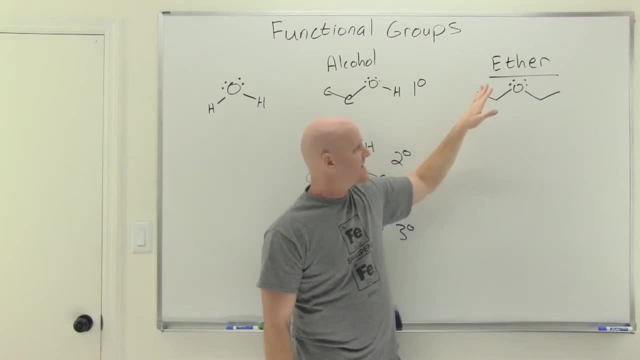 famous member as well, And that's diethyl ether here. So diethyl ether is the one that they used to use as an anesthetic. It'll put people out and stuff like that- And we still use it commonly as a solvent in organic chemistry as well. 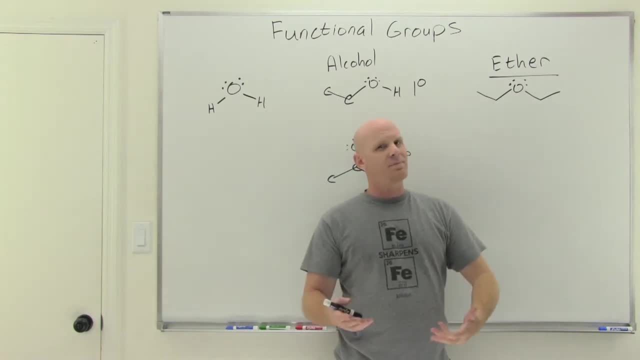 But it's the most famous, And so you know Generically. if somebody just says, hey, pass the ether, Well we know which one they're talking about, But there again are dozens or hundreds of different ethers that could exist. 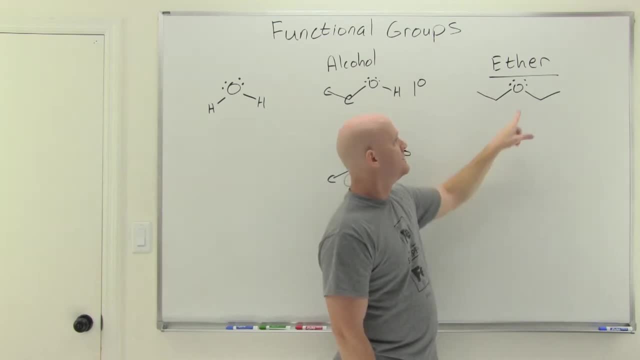 These two carbon chains can be essentially any length carbon chains, But if you have an oxygen bonded to carbon chains on both sides, that is no longer an alcohol, It's an ether. And notice: this guy is not capable of hydrogen bonding as a pure liquid the way an alcohol. 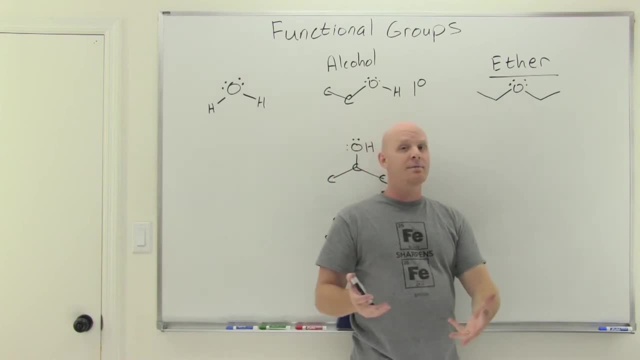 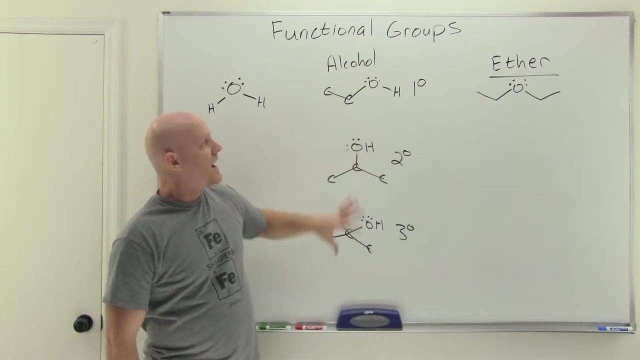 would be, And so it's going to have different physical properties and different chemical properties to the alcohols we just saw. Cool Cool, Let's move on. We'll study the alcohols a lot more than we'll study the ethers, it turns out. 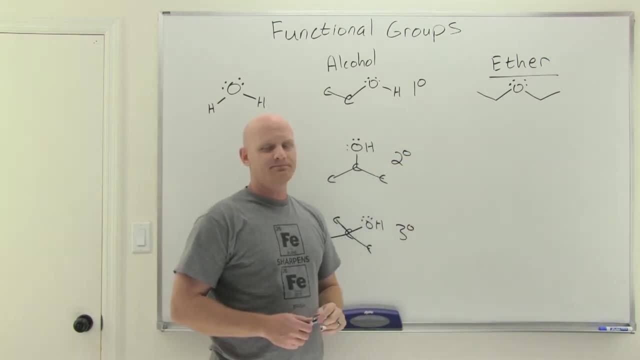 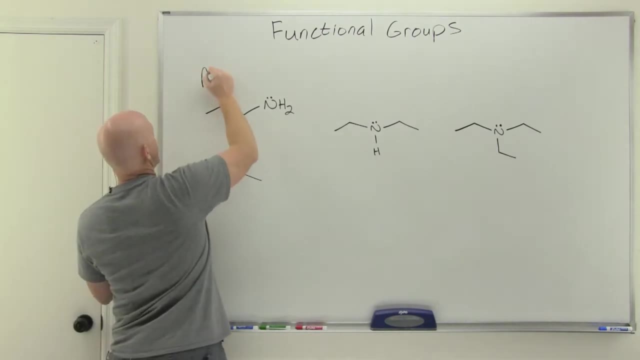 These make great solvents and they don't do a whole lot else, as we'll find out All right. Now we want to move on to a nitrogen containing functional group, And in this case we call these amines So and amines are a little bit unique. 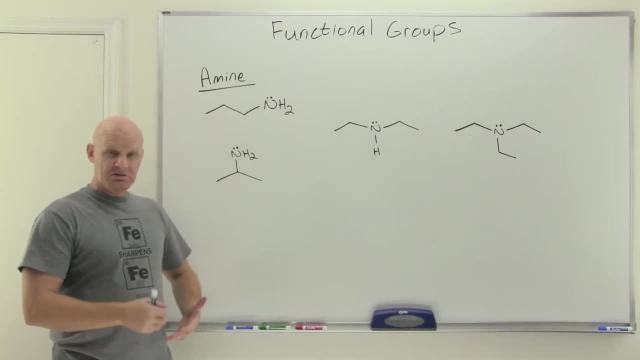 And we won't study these till the very end of second semester. We might, you know, come across one here and there. So, but we classify amines different. Then the rest of the functional groups we've looked at. So again, we looked at you know what: a primary carbon, a secondary carbon, a tertiary? 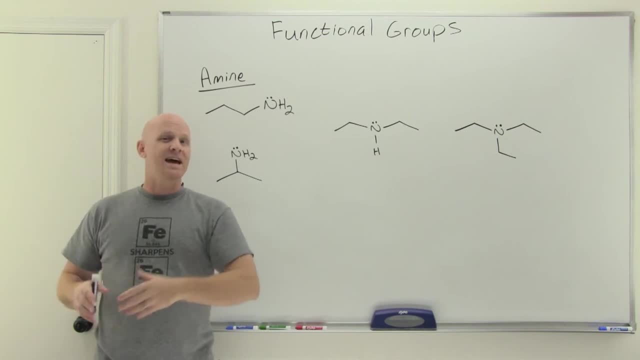 carbon and a quaternary carbon looked like, And we ranked hydrogens and alkyl halides based on the carbon they were attached to. We did the same thing for alcohols, But amines are in principle different, So it turns out for an amine. it's not about how many carbons some carbon is bonded to. 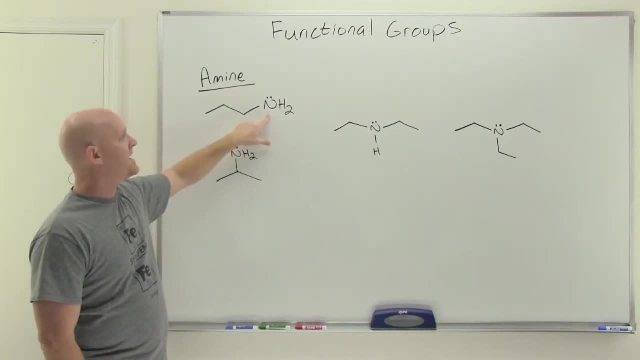 but it's how many carbons the nitrogen itself is bonded to, Because that nitrogen might be directly bonded to only one carbon, like we see in these two examples, And these two would be referred to as protons, Primary amines, Or that nitrogen might be directly bonded to two carbon atoms. 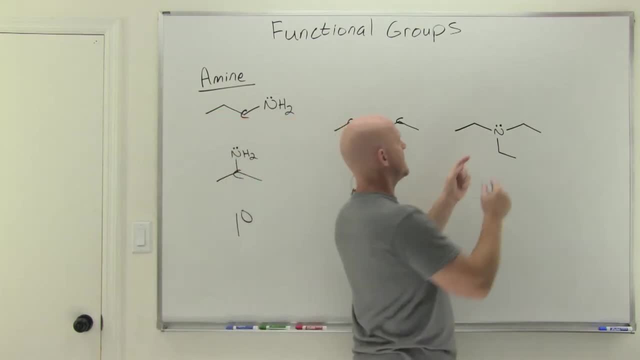 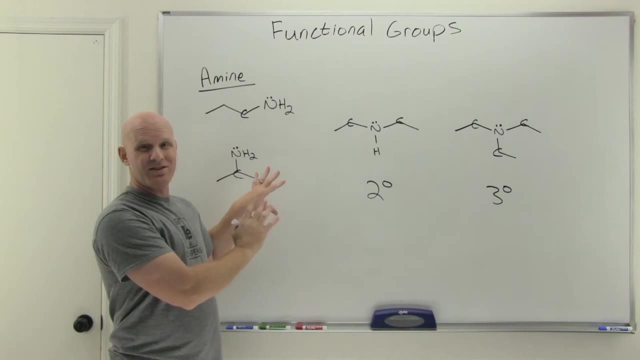 We call this a secondary amine. Or your nitrogen might be directly bonded to three carbon atoms And we'll call this a tertiary amine. So because we classify these a little bit different in how we come out with primary, secondary and tertiary than all the other function groups, students often get a little. 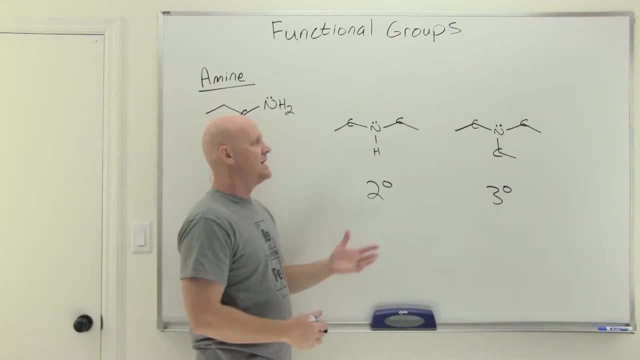 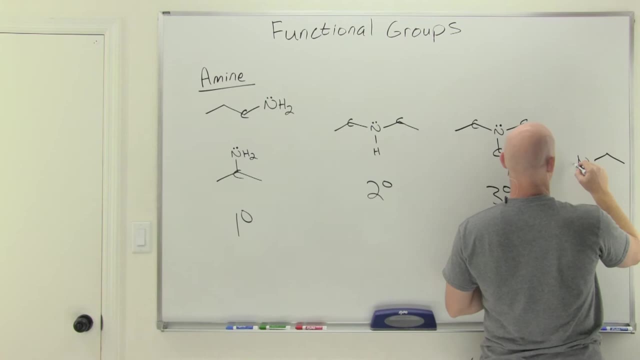 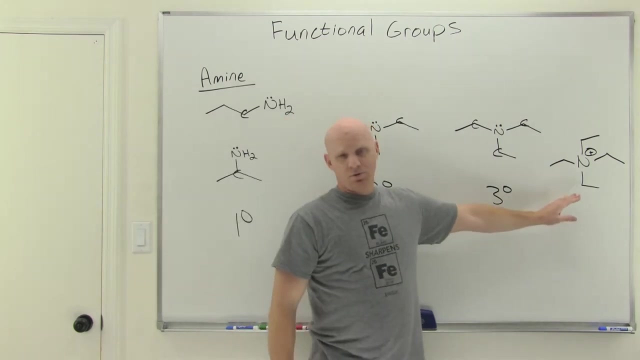 bit confused, So I just want to make this clear from the get-go Now. technically, nitrogen could end up bonded to four carbon chains in certain rare cases, In which case it would end up having a positive charge. So not super important now. 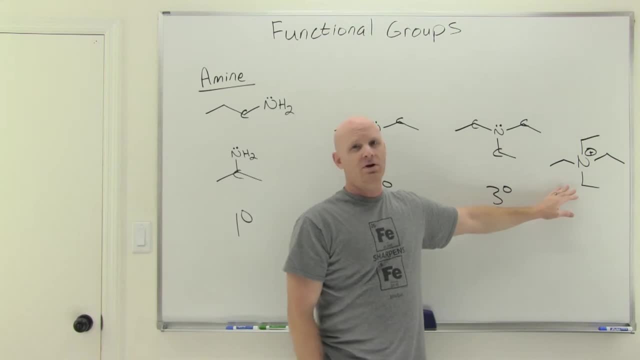 We call these quaternary ammonium ions. You might recall that the ammonium ion is NH4+. Well, this is now a quaternary ammonium ion, So not super important now, But technically I just want to point out that these can even become quaternary as ions. 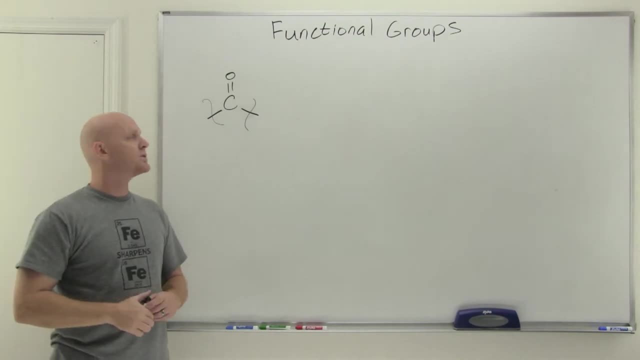 in certain cases. All right. The next couple of function groups I want to look at, In fact the next several, are all going to have a carbon-oxygen double bond. Now I want to point out that a carbon-oxygen double bond can be referred to as a carbonyl. 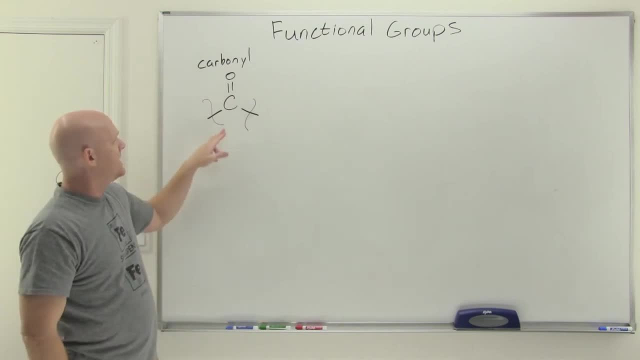 group, or some people say carbonyl whatever, So take it either way, And the question is: what's going to? So a carbonyl itself is not a functional group. It is a part of a variety of functional groups. 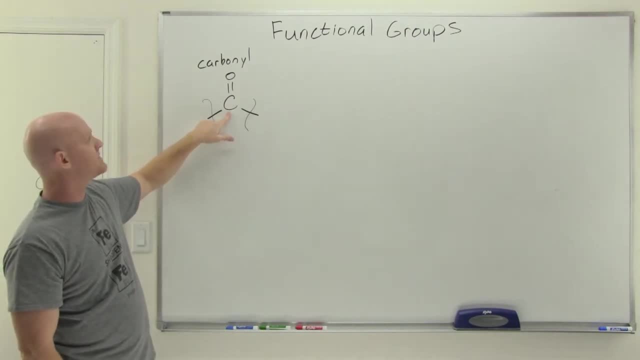 And the question really comes down to is: what is that carbonyl carbon? So we have a carbonyl oxygen and a carbonyl carbon. What is the carbonyl carbon bonded to in these two positions? Now I've, kind of like, showed this squiggly line to show that I've cut those bonds and 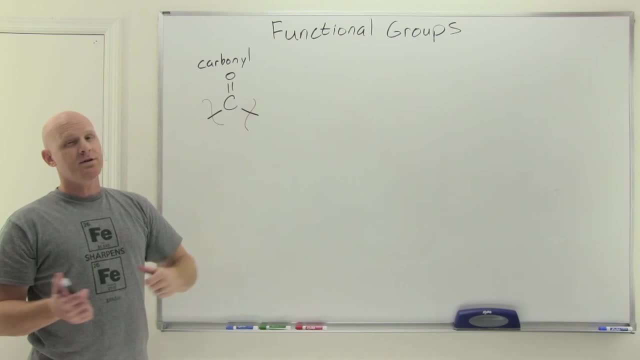 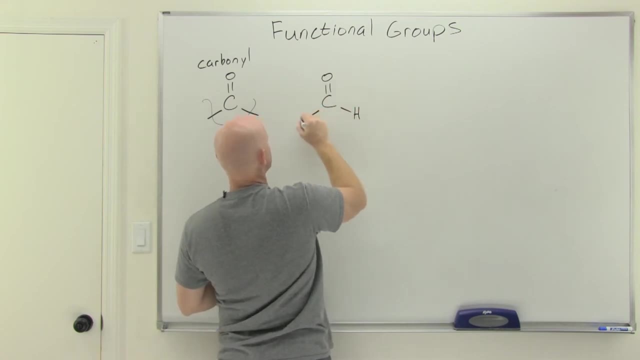 haven't showed you what actually is attached on the other side. But what's going to be attached on the other side will determine the functional group. So we can start. the most basic thing we could have is to just have a hydrogen on both sides. 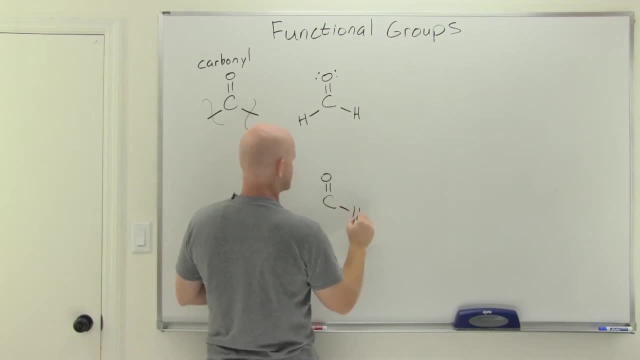 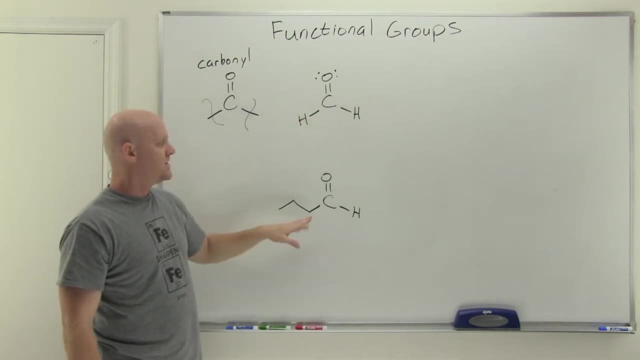 But technically- I'm going to throw this in here- You could have just a hydrogen on one side as well, And in either case this is the only example of one that has two hydrogens on case, but you can have any carbon chain on one side in either of these. 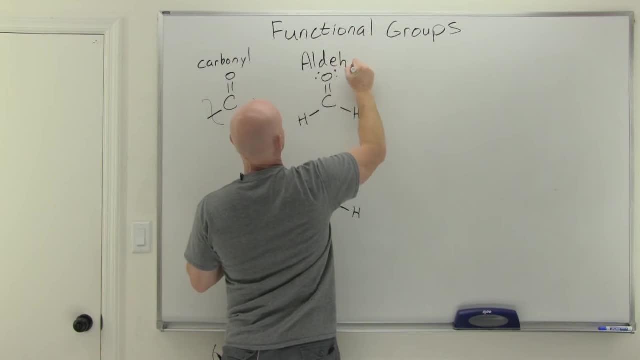 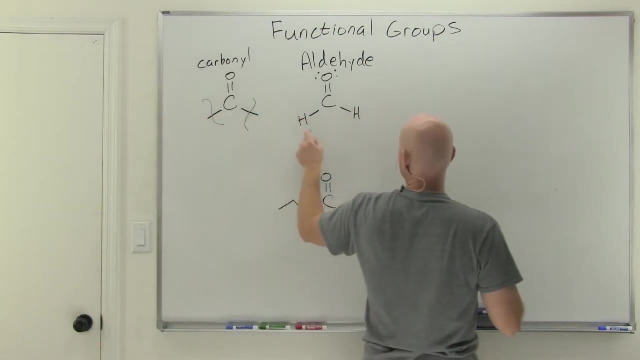 examples. we would refer to this as an aldehyde. So your aldehyde is your first carbonyl-containing functional group. Cool Now if I replace both hydrogens here with carbon chains, instead of just one side of a carbon chain, but I replace both sides with carbon chains. 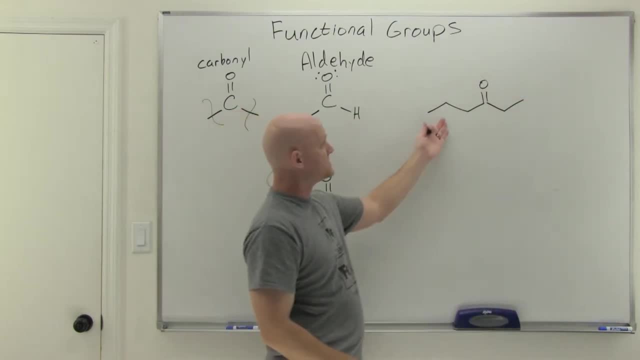 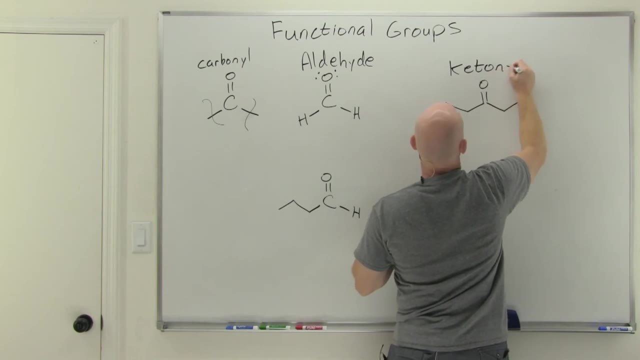 And again, it could be symmetrical. I could have two identical carbon chains or two different ones, It doesn't really matter. So, and in this case, different functional group, And we'll call it a ketone. And it turns out that ketones and aldehydes do a lot of similar. 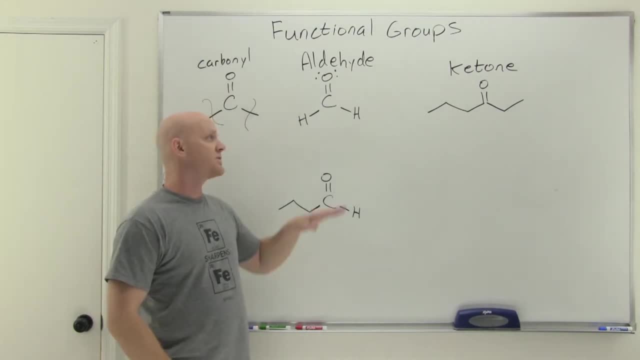 chemical reactions, but they're not identical in certain respects And so they are different functional groups. but you'll find out that when we do a chapter in second semester on chemical reactivity, we'll group these together And the whole chapter will be on reactions of ketones. 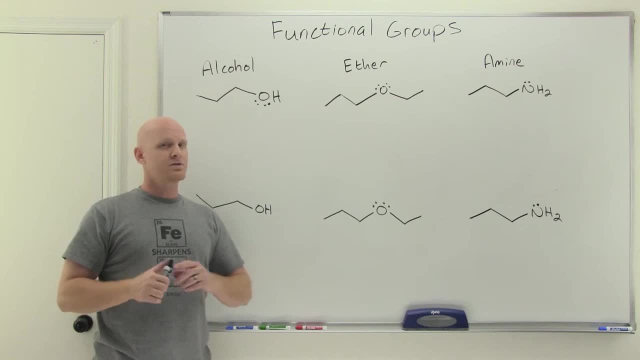 and aldehydes together. All right, I want to cover three new functional groups all at once here, And I put three old ones on because I want you to specifically see the difference between the two, because they're very subtle- And students. 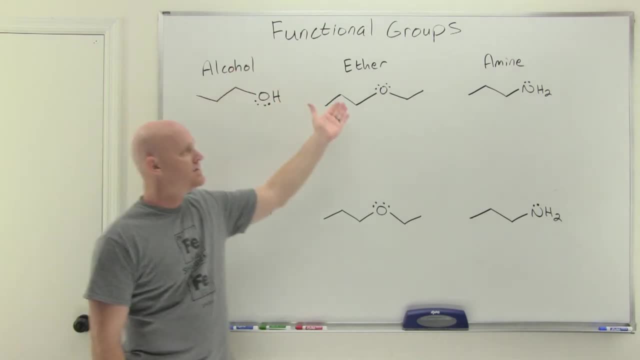 students, especially early on, often don't see the difference. So, but I put alcohol, ether and amine back on the board. Those are still an alcohol, That's still an ether, That's still an amine. And you might be like: well, Chad, you just drew them twice. Well, I'm going to alter. 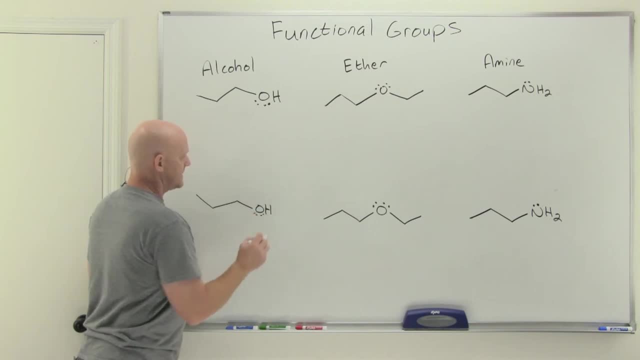 these. Don't worry, We've got a couple of lone pairs on this auction here, So I'm going to alter these just ever so slightly. And so on the carbon attached to the OH, or either carbon attached to the oxygen in the ether or to the carbon, in this case, attached to the nitrogen, I'm going to 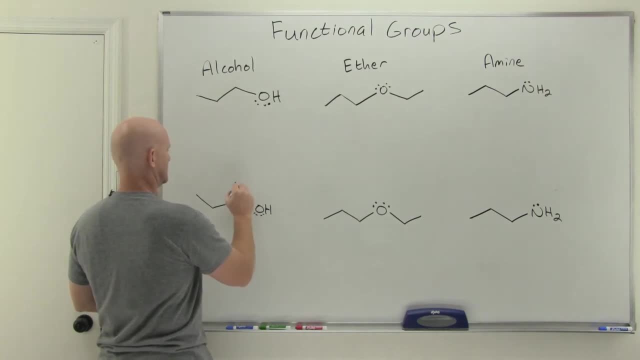 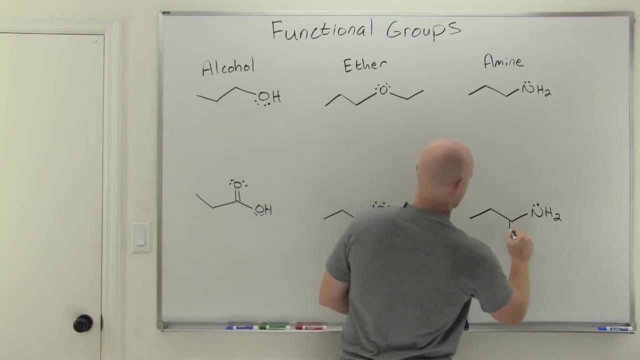 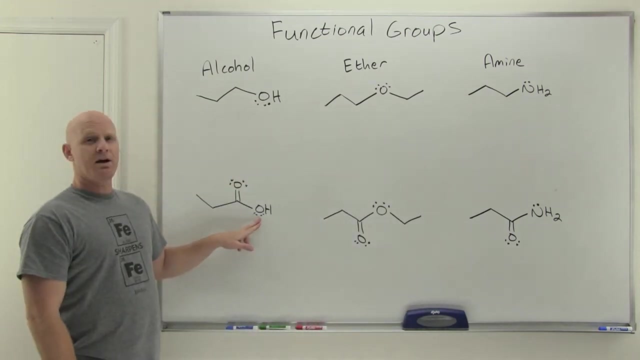 actually add a double bond to oxygen. So there and this I could have done on either side technically and then also here. So and it turns out that when you've got an atom with lone pairs, if those lone pairs are one bond away from, 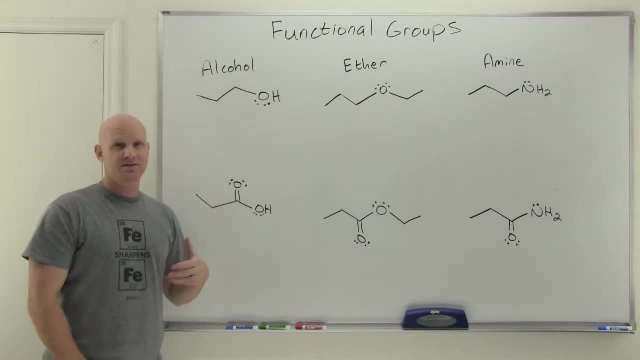 the location of a pi bond, there's going to be resonance taking place and resonance will affect the chemical reactivity and the stability And that's why these are going to actually get classes, different functional groups than the three we saw up top. This is no longer an 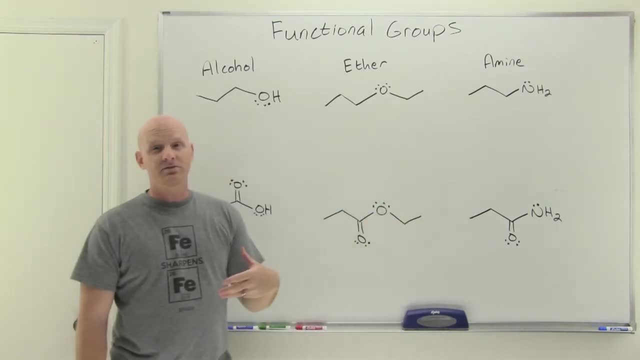 alcohol. This is no longer an ether And this is no longer an amine because of resonance. They actually have different physical properties and different chemical reactivity than alcohols, ethers and amines instead. So if we look here, this first one here is called a carboxylic acid. 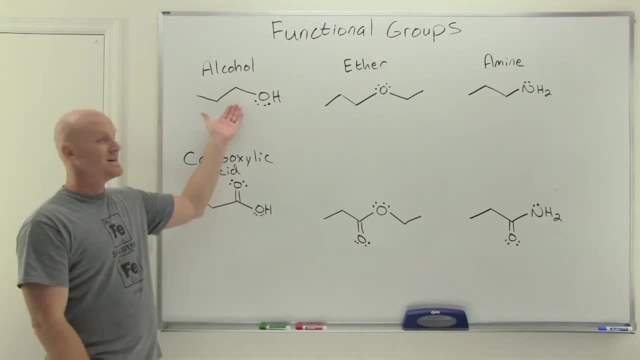 So, and because of resonance, it's much more acidic than an alcohol. So an alcohol is on par with acidity, like with water, but a carboxylic acid turns out acidic acid, like in vinegar. So much, much, much more acidic due to resonance it turns out. So this next one here is called: 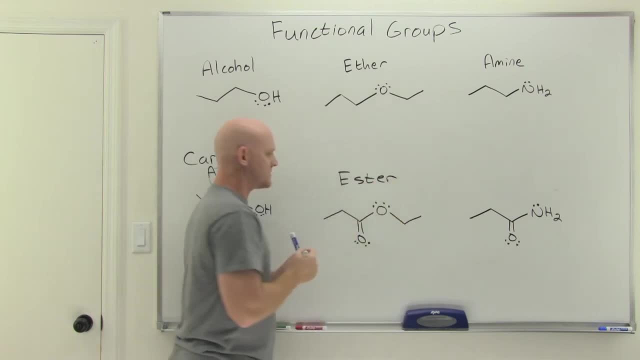 an ester, And so this one's tricky. This is the one that students often get fooled by. So because we have ether and we have ester and even the names kind of look very similar and stuff like this. So but once again you have resonance and esters undergo quite a few chemical. 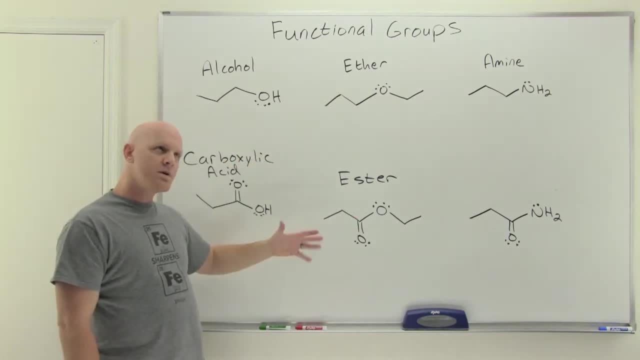 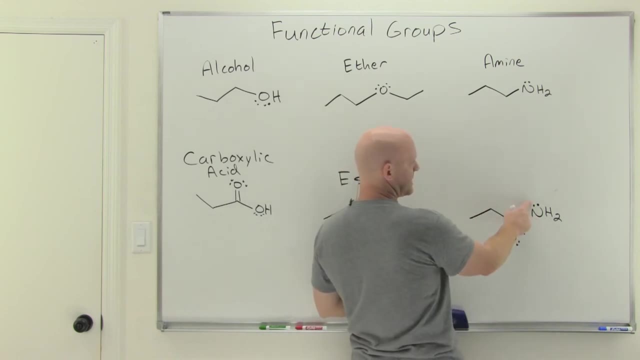 reactions that ethers never do. Again, it can sort of be related to resonance. It's not quite simply a resonance thing in this case. So same thing here. We've got resonance, that lone pair on the nitrogen, so it can be associated with the oxygen here. And 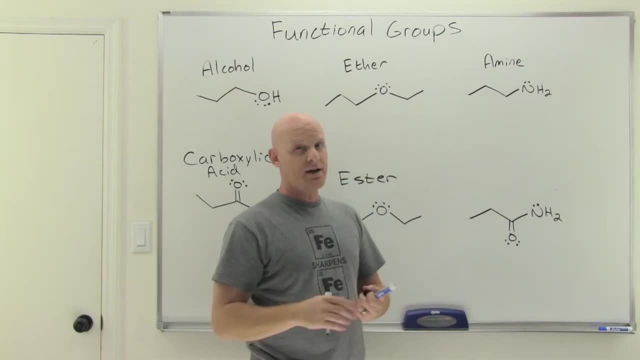 so, whereas amines are actually pretty decent organic bases, they act as bases. amides are not basic at all, And that's what this is called an amide. And so, once again, resonance changes this to have a slightly different chemical and physical behavior, And so we give it its own distinct. 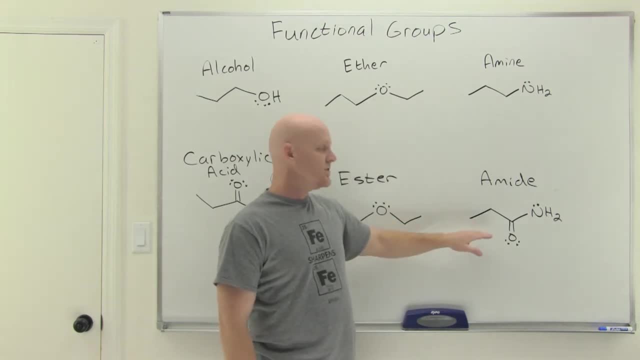 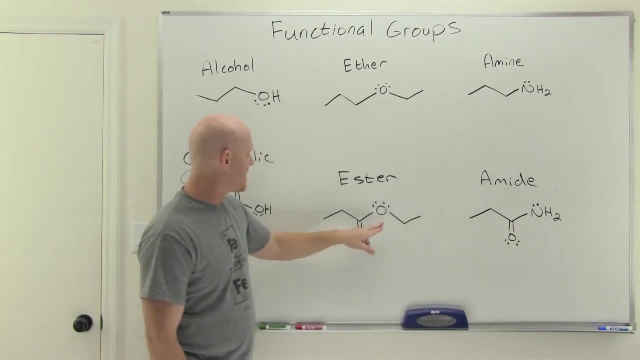 functional group. So these are amines. this is an amide. Note the difference And note where you put that carbon oxygen to the wand has to be immediately adjacent To the nitrogen here, or the oxygen here, or the oxygen here If you put it further away. 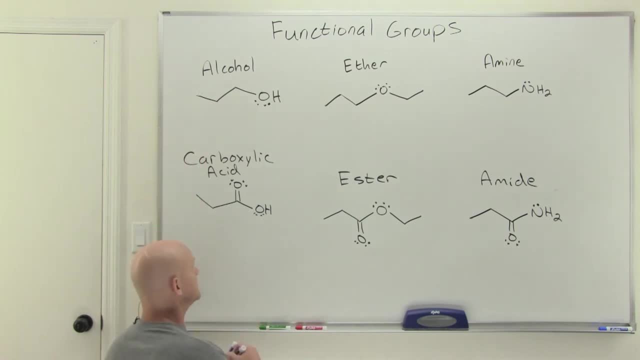 you actually don't have any of these functional groups. So, for example: So let's say I put the OH there, but I put the double bond oxygen either here, here or here. I had to put it there to make it a carboxylic acid. Well, in this case, 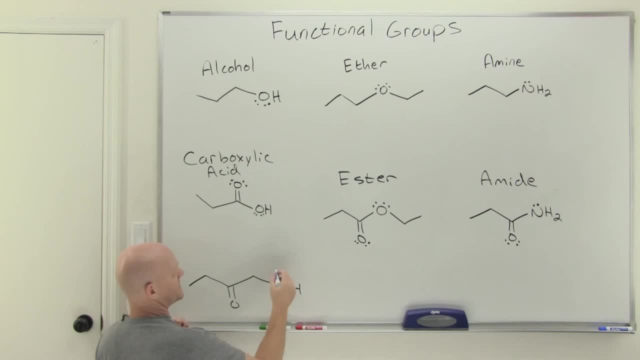 these would actually just be two different functional groups. This one over here would actually still just be an alcohol And this over here a carbon double bonded oxygen bonded to two carboxylic acids. And so we have this double bond oxygen here to bond this carbon double bonded oxygen. 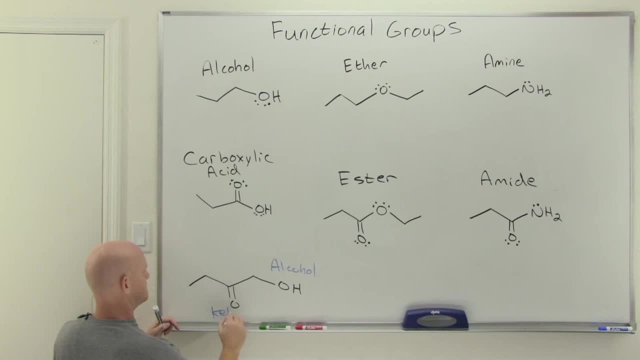 carbons on either side. that would be a ketone, Cool. And so nothing says you can't have multiple functional groups in the same molecule. In fact, one of the more common types of problems you're going to get on this stuff is they're going to give you some giant molecule and then they're 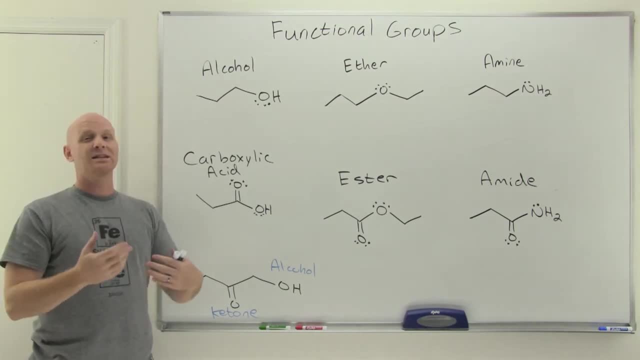 going to want you to circle every functional group that's present in the molecule and label it appropriately. Well, this one here has got two different function groups: an alcohol over here and a ketone over here. But this one over here just the one function group and it is not an 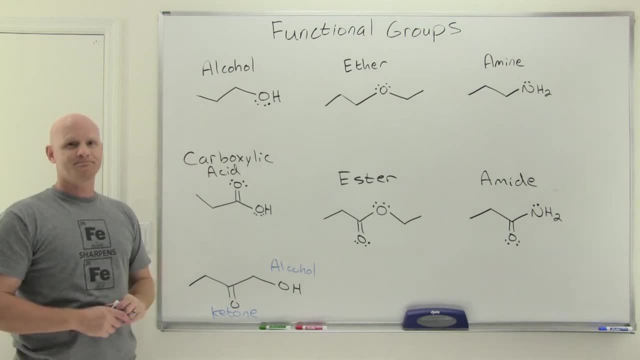 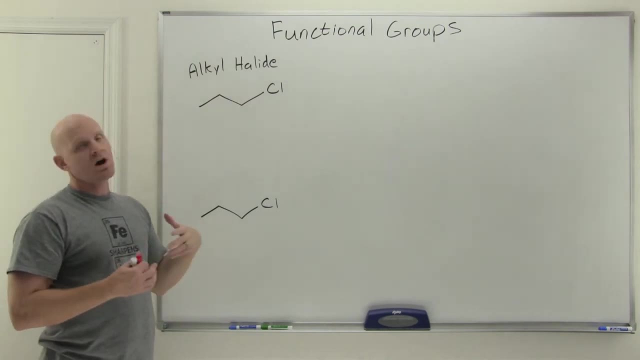 alcohol, so it is a carboxylic acid instead. All right, just wanted to bring back up an alkyl halide And, in similar fashion to how we saw, if you put a carbon-oxygen double bond right next to the OH, where you normally think you have an alcohol, it's a carboxylic acid. now, Same thing. 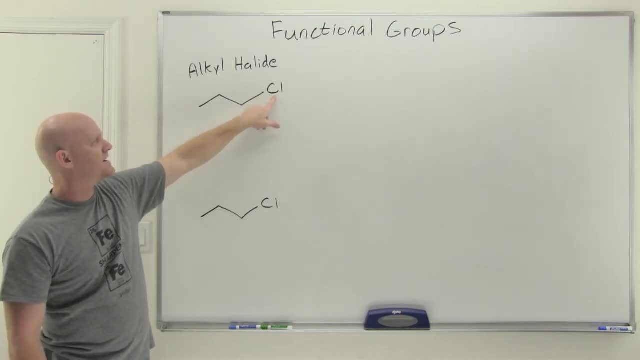 here We call this an alkyl halide and the atom directly. the carbon directly attached to the chlorine is sp3, hybridized and alkane-like. so that's an alkyl halide. However, just like before, if I take that carbon instead and give him a double bond to oxygen, 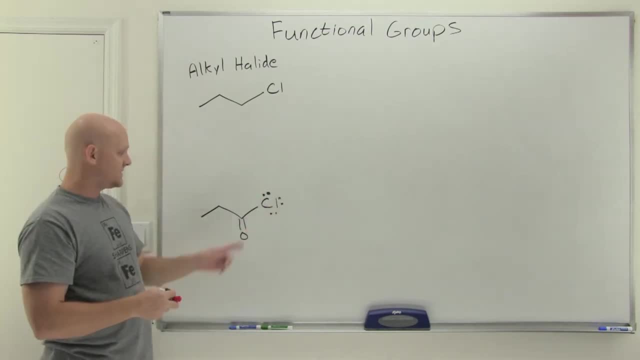 well then, the lone pairs on chlorine are once again going to have resonance with the oxygen and it's going to give this some chemical reactivity that wasn't present up here. So these don't have the same chemical properties and don't do the same kind of chemical reactions, And 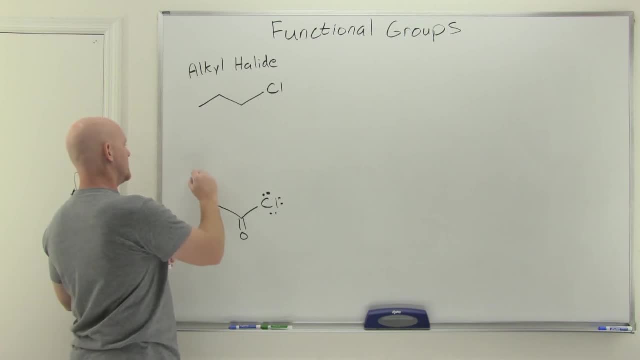 as a result, this gets its own functional group name. Instead of being an alkyl halide, we would refer to this as an acyl halide, So, and some people even call it an acid halide. so because it turns out it can be derived. 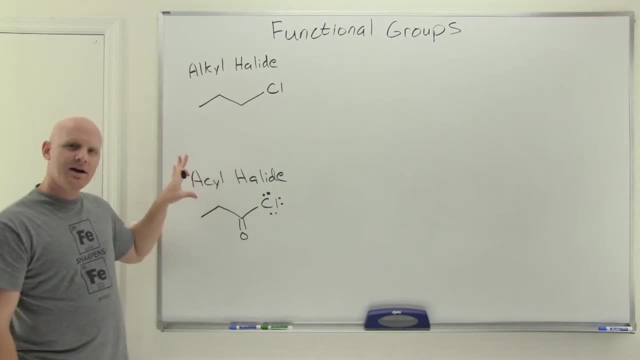 from a carboxylic acid as well, But acyl halide or acid halide, that's what this guy is. And again, the key is that the carbon that's double bonded to oxygen has to be the one bonded to the halogen. 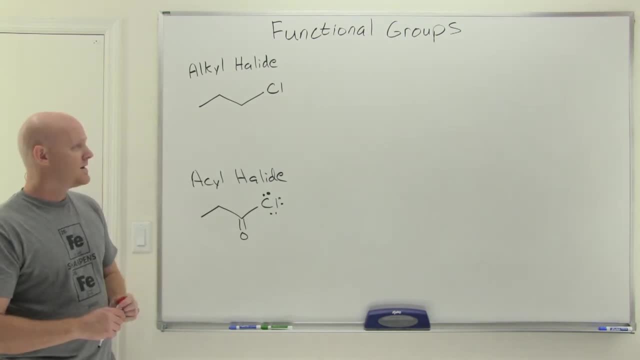 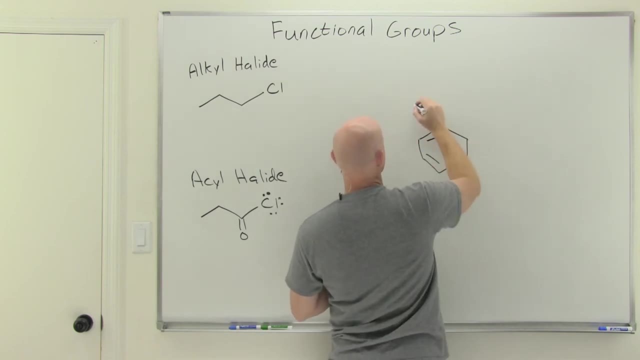 for it to be considered an acyl halide. All right, we've got one last other to cover, and that is when you have this lovely structure here. Now it turns out this compound right here is just simply called benzene. That's its name. 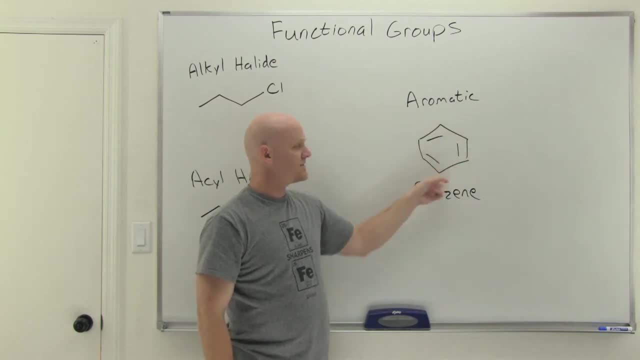 So that's benzene, Benzene, And it looks like you've got, you know, six carbons in a ring and it looks like you've got alternating double and single bonds all the way around. But it turns out, due to resonance, it turns out there's delocalization of the pi electrons, all the 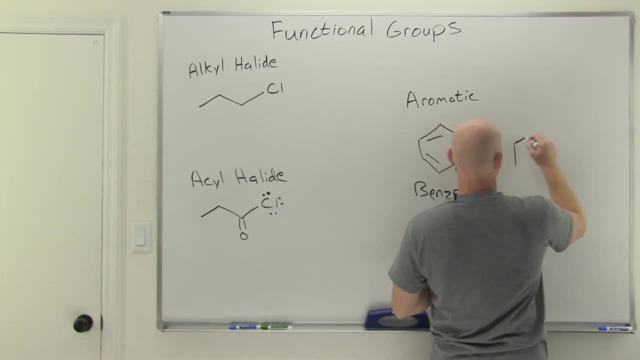 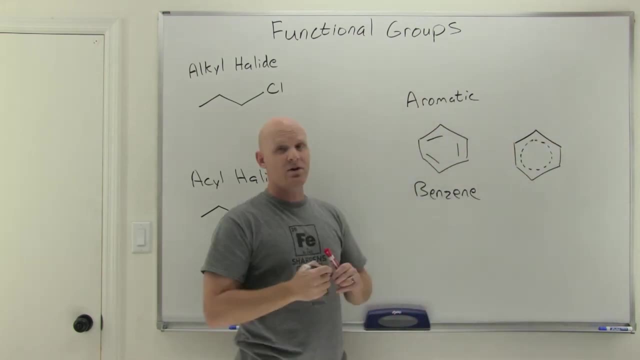 way around the ring, And so another way we might draw this is like: so just to show that delocalization there, It turns out there are no double bonds or single bonds in a benzene ring. They're essentially like the equivalent of one and a. 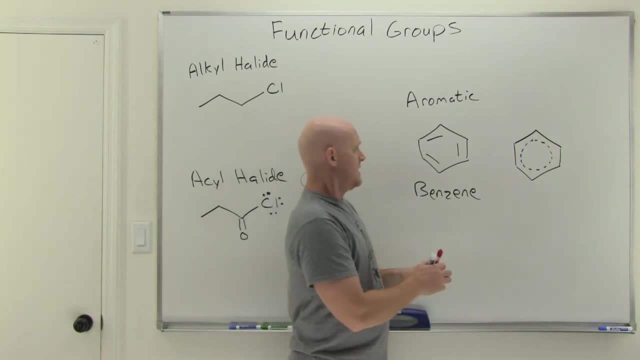 half bonds all the way around, Cool. So sometimes we end up drawing this and we just draw a hexagon and we get lazy and we put a circle in it And that's another way of representing a benzene ring as well. Now it turns out benzene. 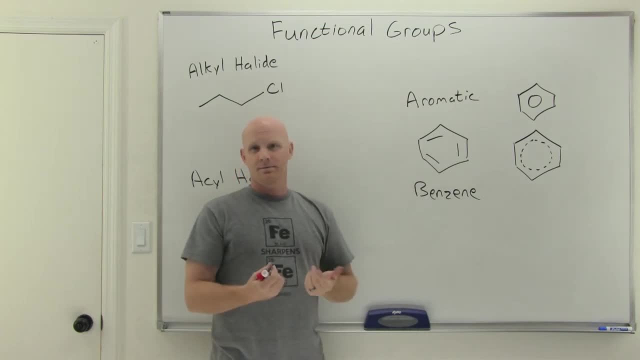 is by far the most common aromatic compound out there, by far. So- and again, you can attach other stuff to it. So put other different things on there and stuff like that, And this would still be considered an aromatic group. Cool, So now you know how to draw a hexagon, So let's go ahead and 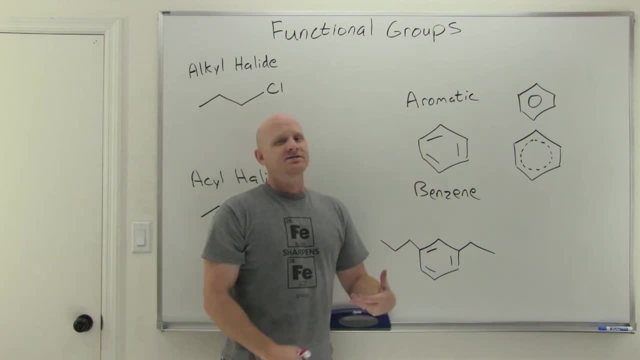 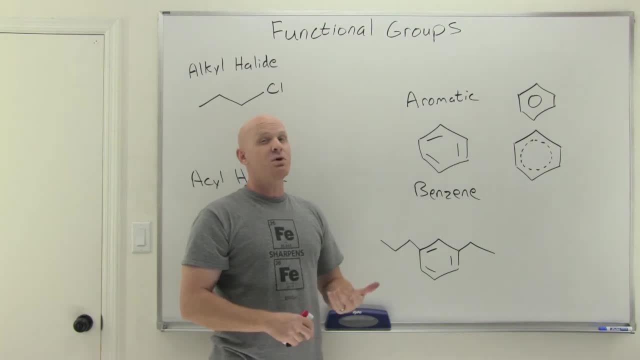 benzene rings are not the only aromatic compound out there, just the most common by far. We'll find out that other rings and stuff like that have a chance of being aromatic, but that's really complex And we'll have a whole chapter to talk about that. So and learn those things, But for 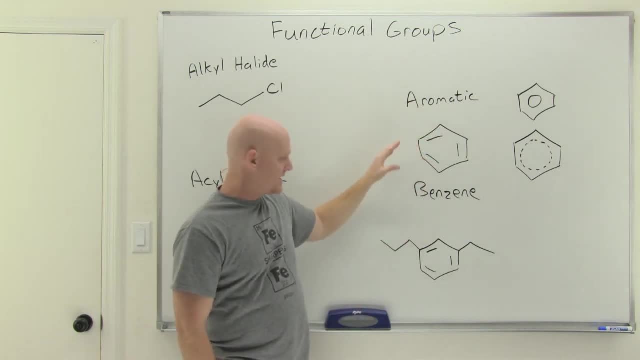 now. just think of benzene and anything containing a benzene ring as being your classic aromatic compounds. All the other types that are much less common, we will study those in second semester. Don't worry about them now at all. Cool, Like I said, there are other functional groups that exist out there and stuff like that.